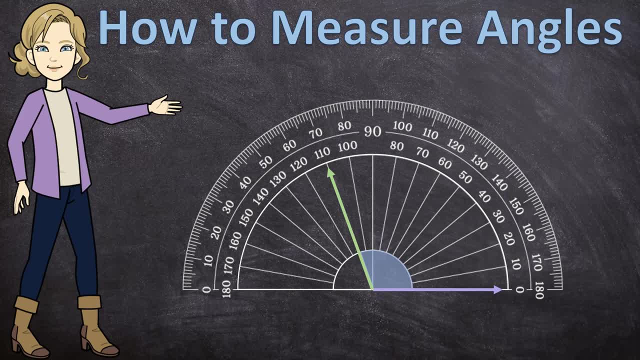 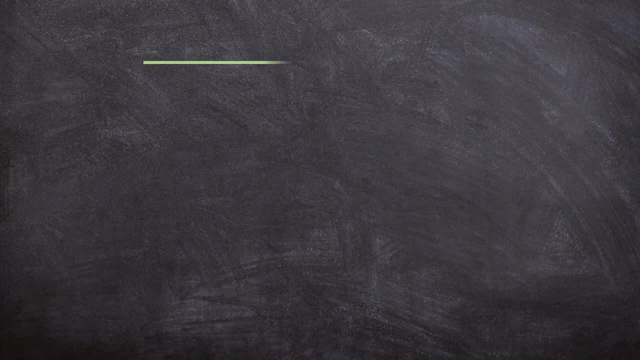 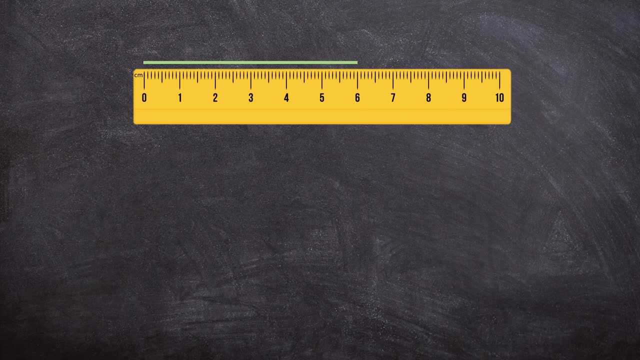 In this video, I'm going to show you how to measure angles using a protractor. So hello everyone and welcome to Mathematics with Marleen. When we have a line, we can easily measure this line using a ruler. For instance, this line is six centimeter long. But what if we have two rays and we want? 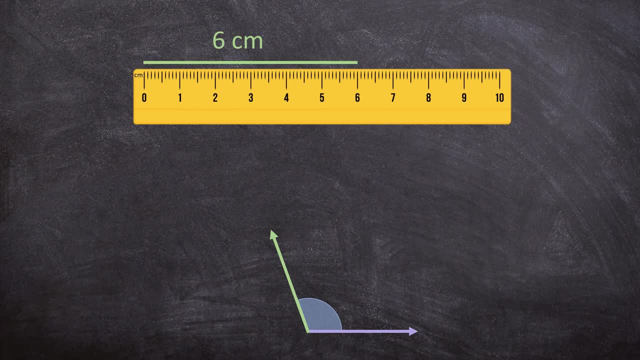 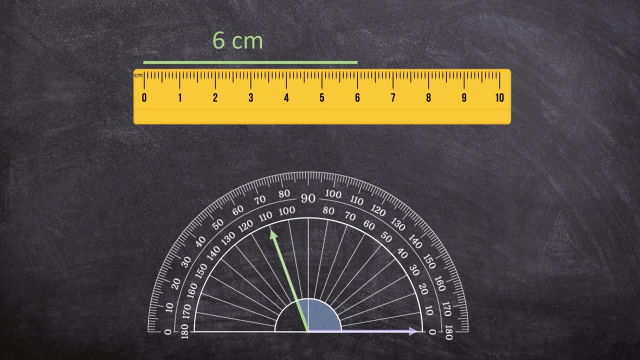 to measure the angle between these two rays. Now we can't use a ruler anymore. We need to use a protractor to measure this angle. And this angle is 110 degrees, And degrees is the unit in which we measure angles, So always remember the degrees. But how do I measure angles? Let me show you. 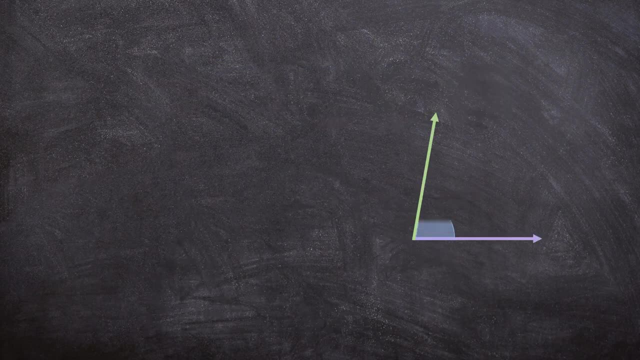 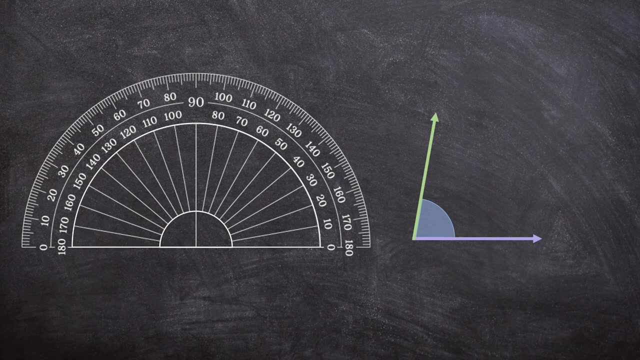 Here we have two rays and we want to measure this angle between the two rays. So first we need our protractor And then there are two things I want you to remember before you measure your angle. The first thing: can you see in the middle, at the bottom of your protractor, There's that T, This 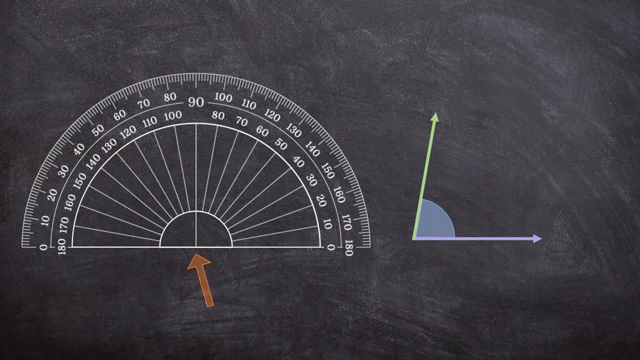 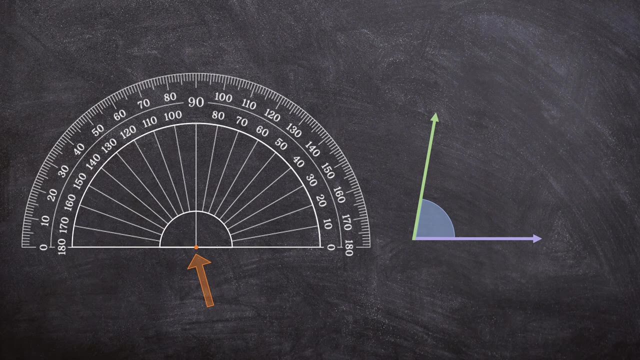 may look different on different protractors. Sometimes there's a dot, Other times there's just this T And other times there's a little hole to indicate this space. But all I want you to remember is to line up the bottom middle part of this protractor with the vertex of the angle. 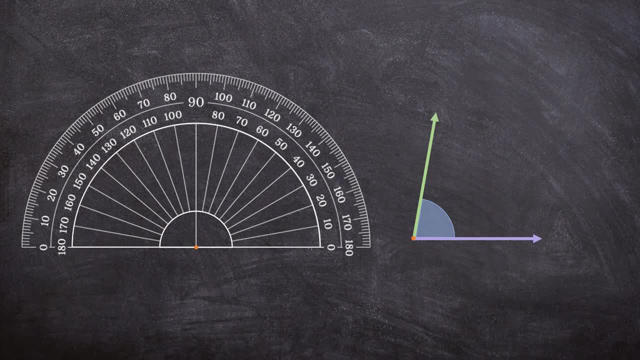 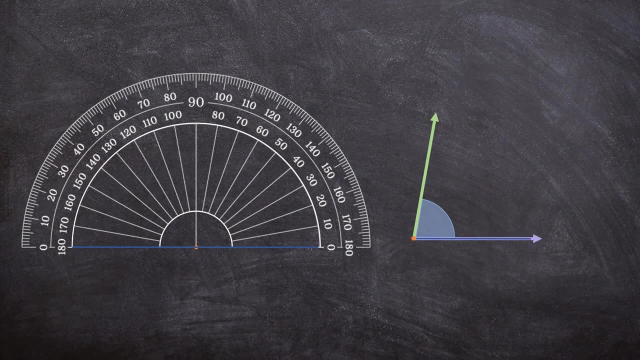 And the second thing I want you to remember is to line up this bottom horizontal line of the protractor with one of the rays. So let's follow those two steps before we measure the angle. So first we line up the middle bottom part of the protractor with the vertex And then we make 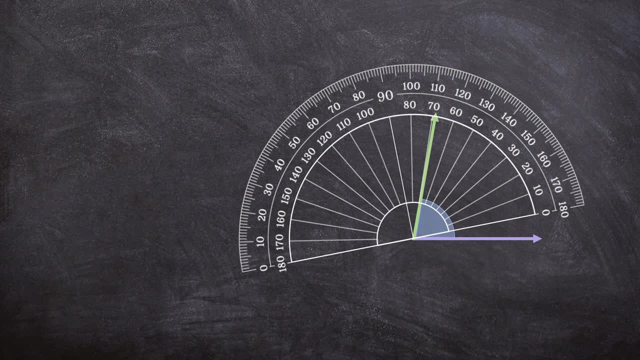 sure that the bottom line of the protractor lines up with one of the rays. I chose the purple ray, And now we can measure the angle. And the second thing I want you to remember is to line up the protractor with the vertex of the angle. So let's follow those two steps before we measure the angle. 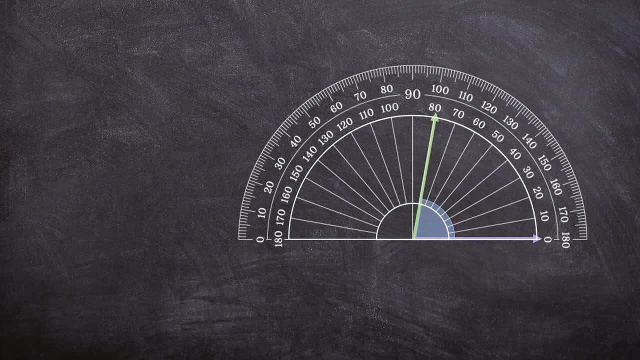 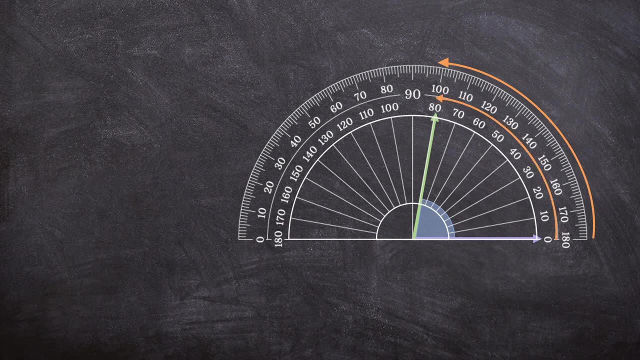 But before we do that, are we going to use the outer numbers to measure the angle, Or are we going to use the inner numbers to measure the angle? You always want to start at zero. So in this case, because our purple ray is pointing at zero here, we are going to use the inner numbers. 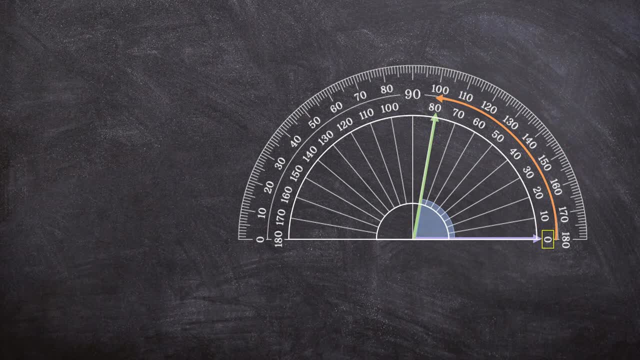 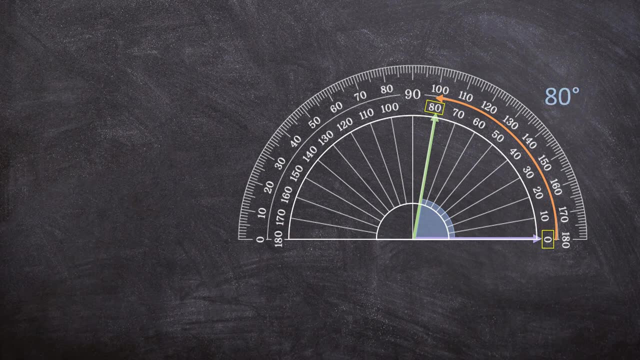 And now we can measure the angle. So our purple ray is at zero And our green ray is at 80 degrees. So this angle is exactly 80 degrees, And always make sure to remember your degrees. It's not just 80,, it's 80 degrees. But how about this angle? We want to measure this angle between: 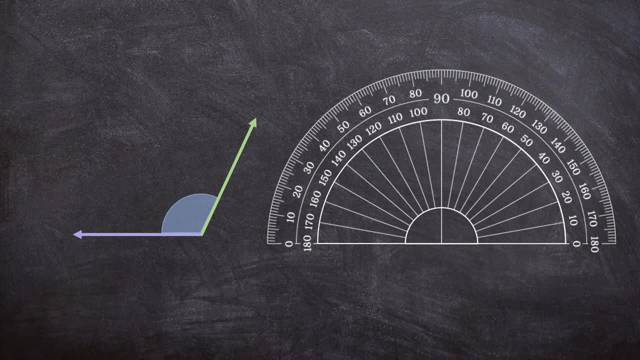 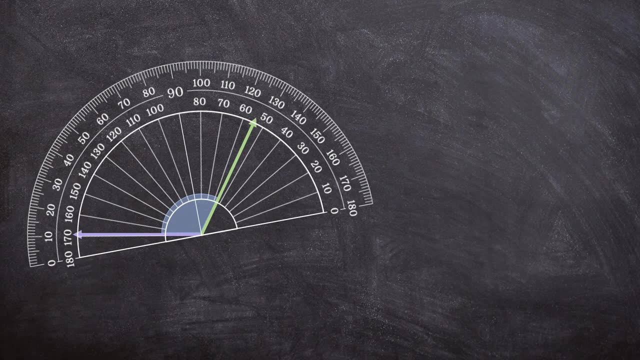 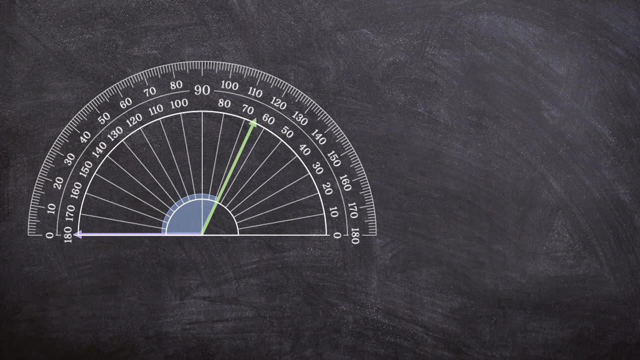 these two rays. First we line up the bottom middle part of the protractor with the vertex of the angle And then we make sure we line up the bottom part of the protractor with one of the rays And now we can measure the angle. But now do we use the outer numbers Or do we use the inner? 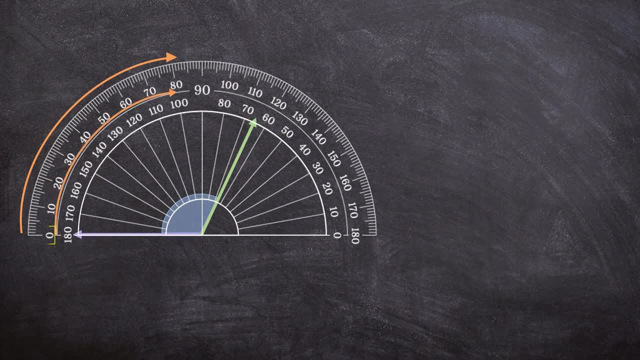 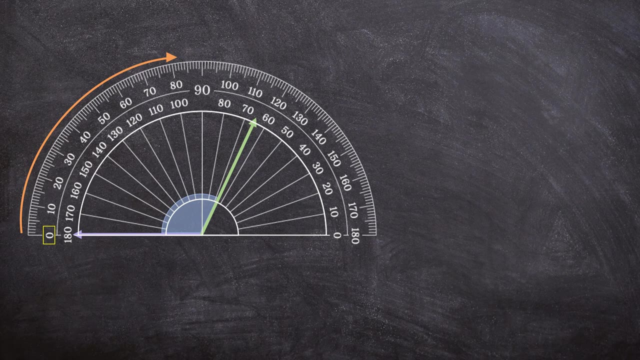 numbers again. Remember, we want to start at zero And our purple ray points to the zero on the outer numbers. So we are going to use the outer numbers And now we can measure the angle. So our purple ray is at zero degrees And our green ray is at 115 degrees, But now we can measure the angle. 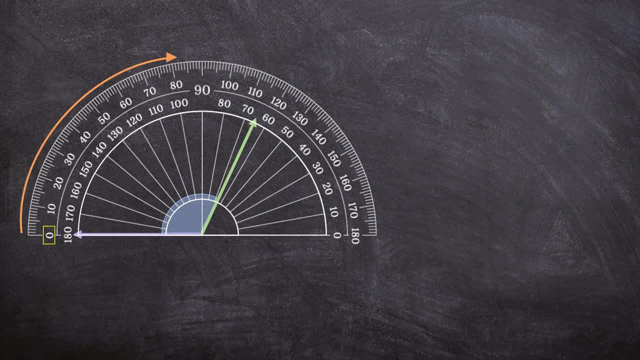 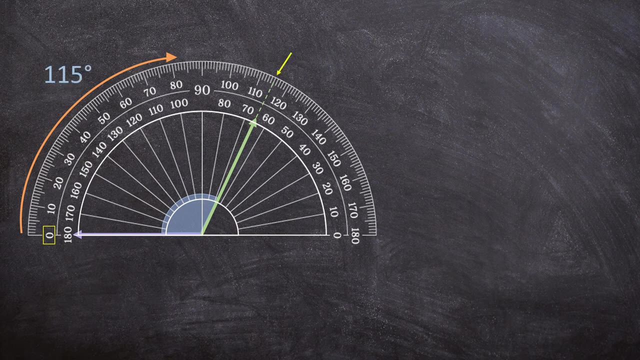 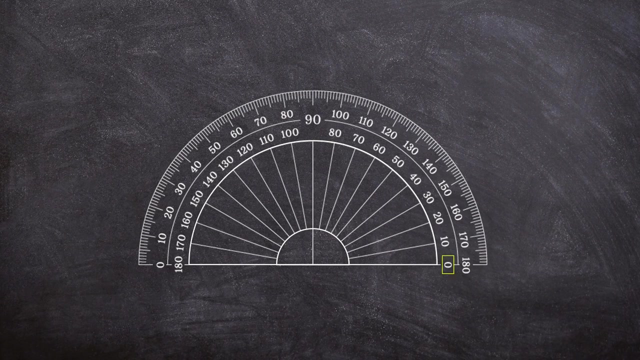 if you can't see clearly that your ray is pointing at 115 degrees, make sure you extend that ray so that you can see exactly to where the ray is pointing. and it is pointing at exactly 115 degrees. but sometimes we can have another problem: our protractor only measures from 0 to 180 degrees. 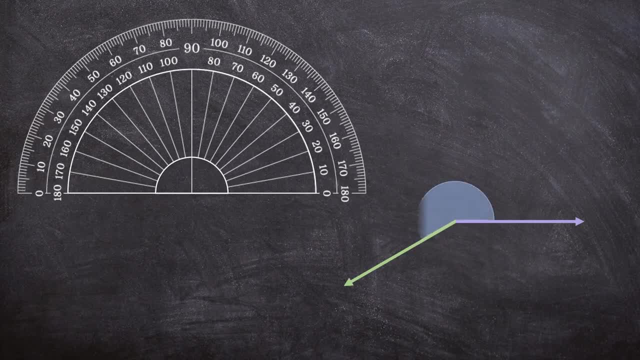 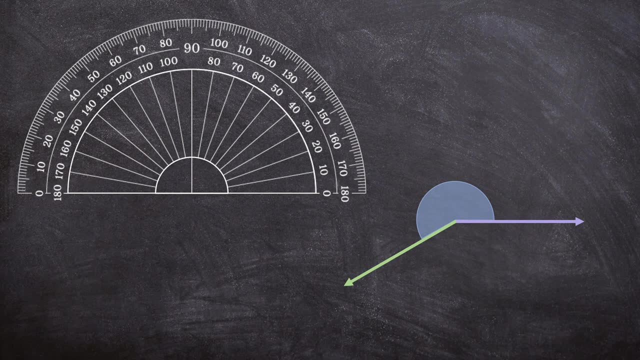 but what if we have an angle that's bigger than 180 degrees? how will we measure this angle? we can still very easily measure this angle. the first thing we're going to do is we're going to measure 180 degrees, and then we're going to measure the rest of the angle and add these two together.